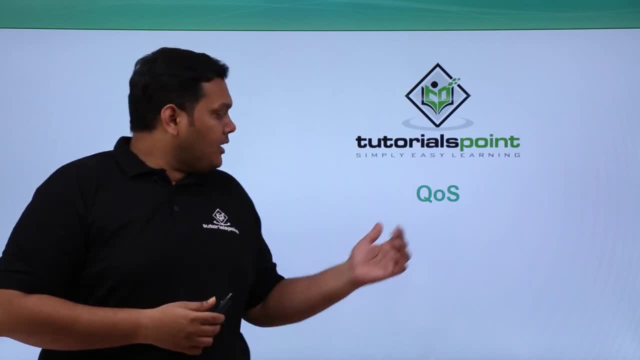 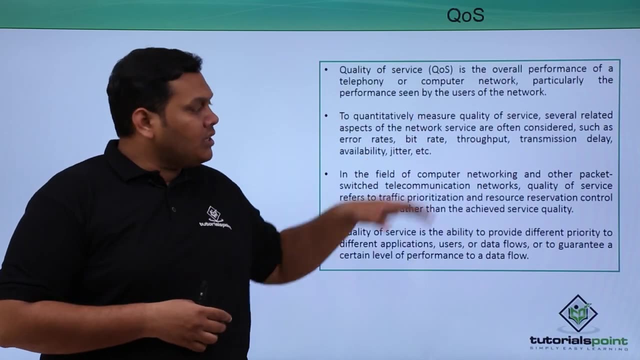 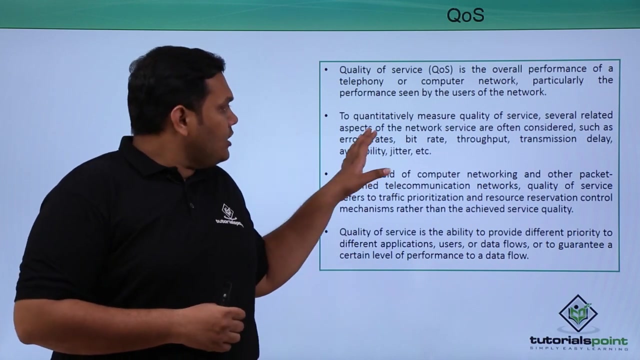 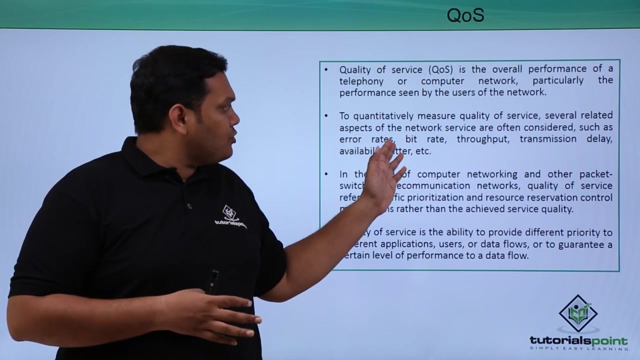 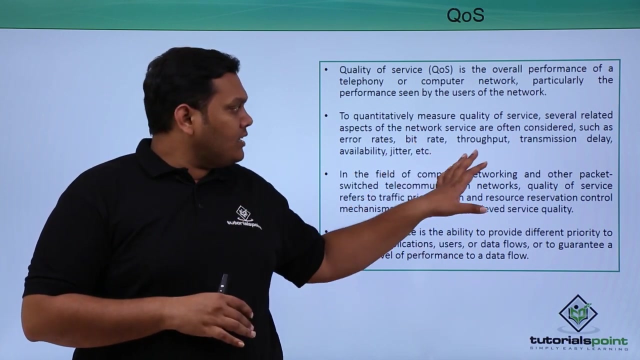 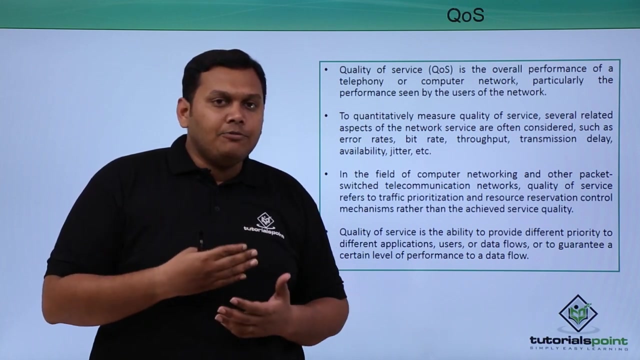 In this video we are going to discuss about the QoS. QoS is Quality of Service. It is the overall performance of the computer network and particularly it is about the performance seen by the users who are using the network. So here to quantitatively measure the quality of a service, there are several related issues in it. So the several related aspects or issues of the network services are often considered and such as error rates, bit rates and also regarding to the thorough outputs, transmission delay rates and also the availability and etc. are considered for the thorough performance of the computer network. 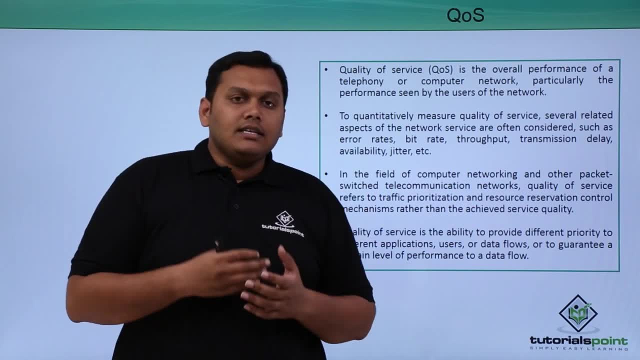 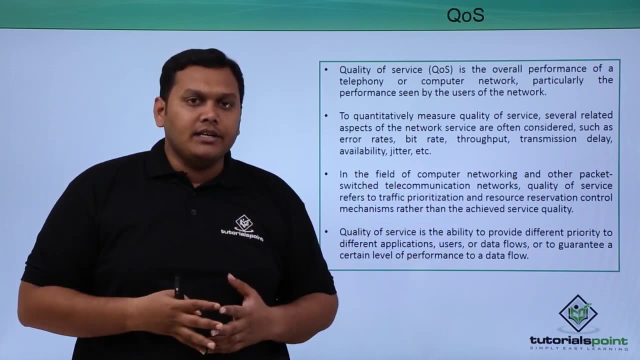 And here in the field of computer networking we can have a package of QoS So we can have a packet tracer and also you can see packet switching. communication networks are also should be monitored so that we can give the quality of the service to the users who are using the network. 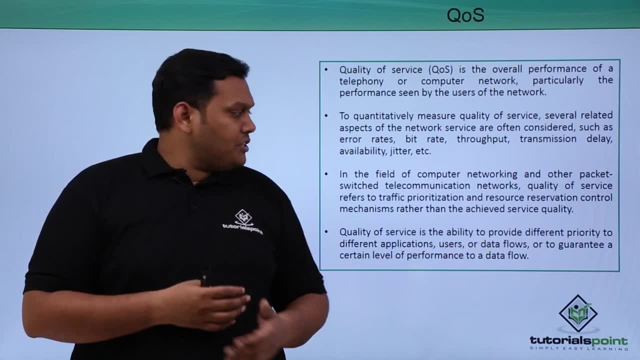 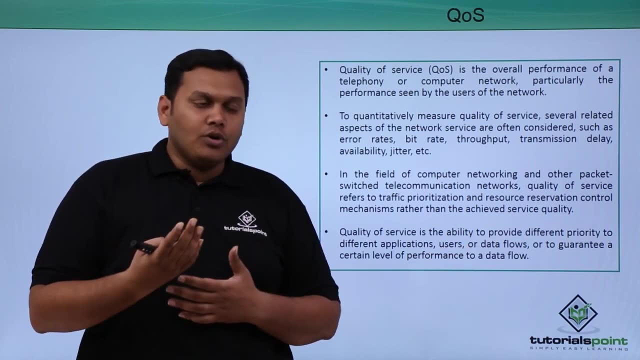 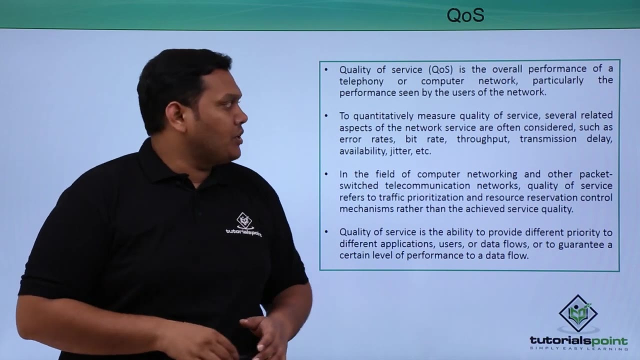 So quality of the service is the ability to provide the differentiation in between the priority, different applications and also here the applications which are used. the users who are using and also the data flows are to guarantee how the packets are not being dropped in between the network. 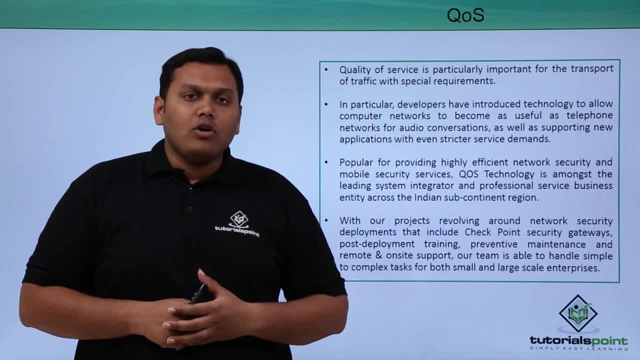 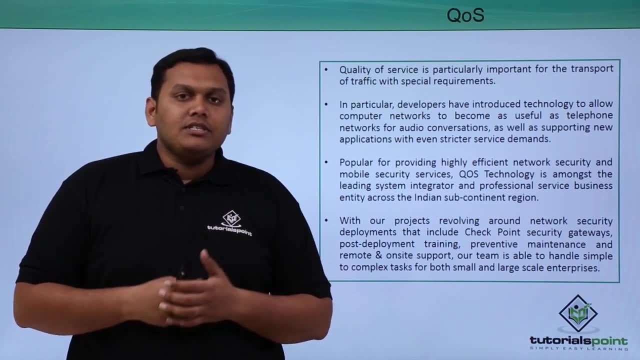 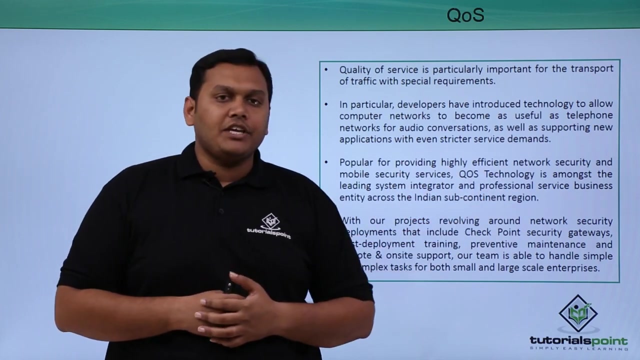 So coming. So the quality of service is particularly important in the transport of traffic with specific requirements and also, you can see, the developers are recent times are creating a new technologies so that we have full support towards this quality of a service for providing the better service for the computer network and also popular for providing high, efficient network. security also is more important in this QoS service. 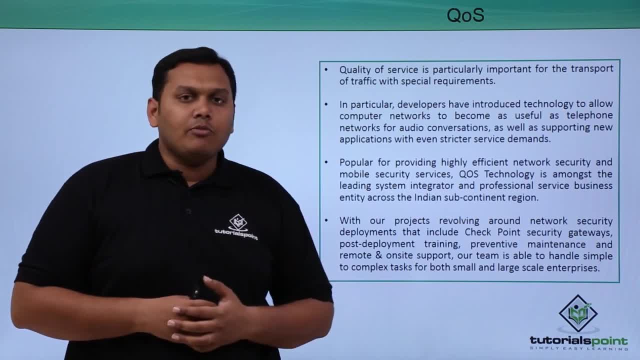 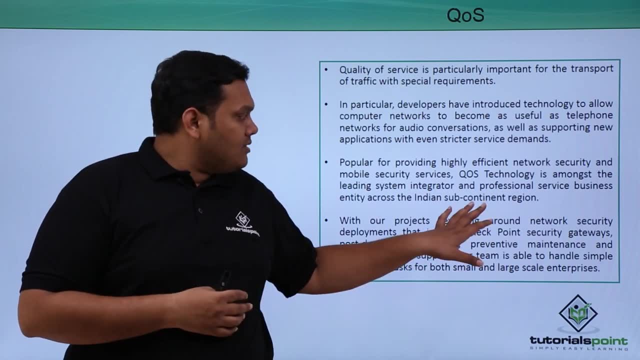 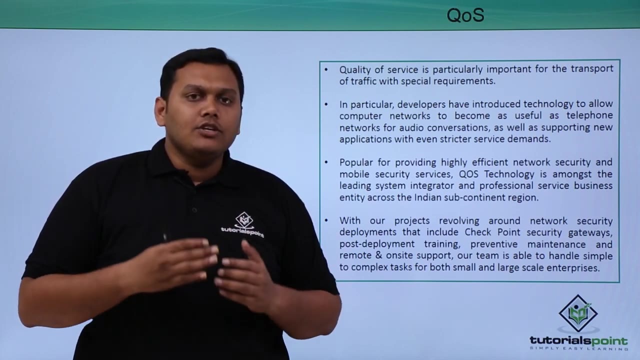 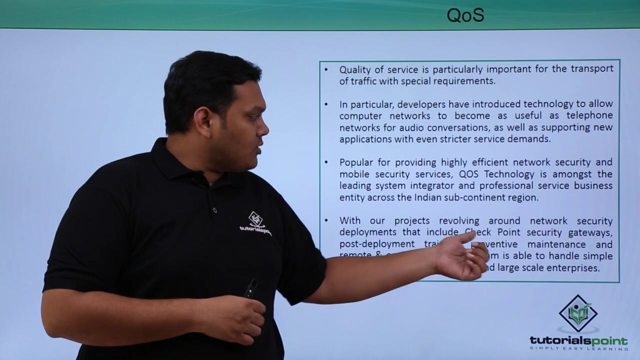 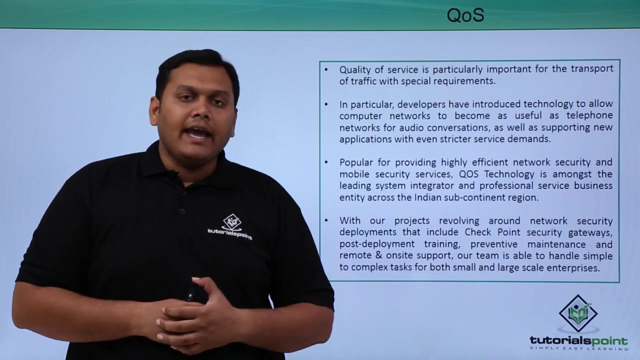 And you can see the QoS technology. I see you can see it's leading Diskussion as it runs through the best computer network and core security. So it needs, So it has, a secure network Establish for the users who are using it. And also you can see the projects following around the network security concepts. here You can see the checkpoint security gateways, Post deployment training And also preventive maintenance. while any operation is not fully prepared, then it needs to be good enough, Definitely.